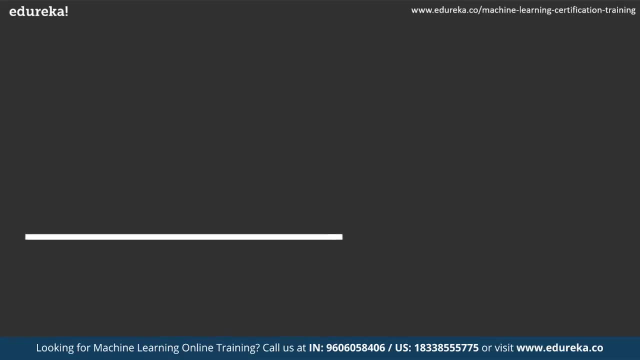 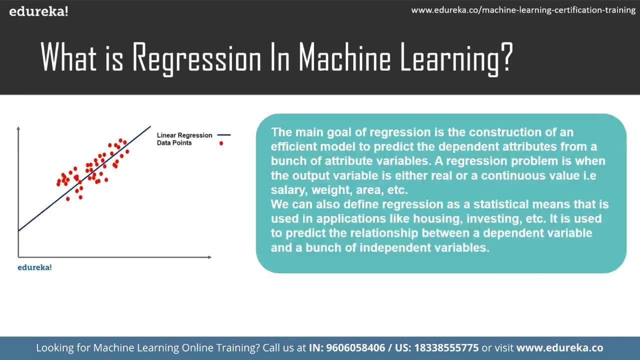 The link is given in the description box below. now, without wasting any more time, Let us understand what regression in machine learning is. So what exactly is regression? The main goal of regression is the construction of an efficient model to predict the dependent attributes from a bunch of attribute variables. a regression, 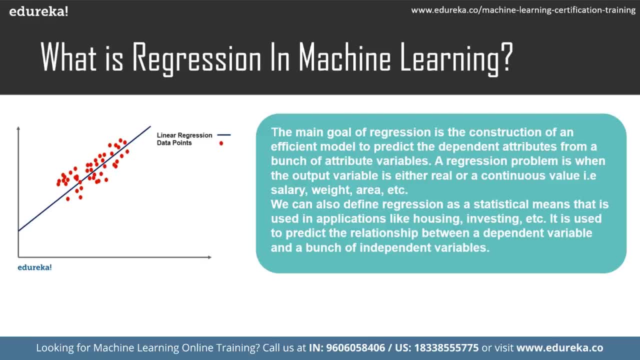 problem is where the output variable is either real or a continuous value, like salary, weight, area, Etc. We can also define regression as a statistical means that is used in applications like housing investing, Etc, to predict the relationship between a dependent variable and a bunch of independent variables. 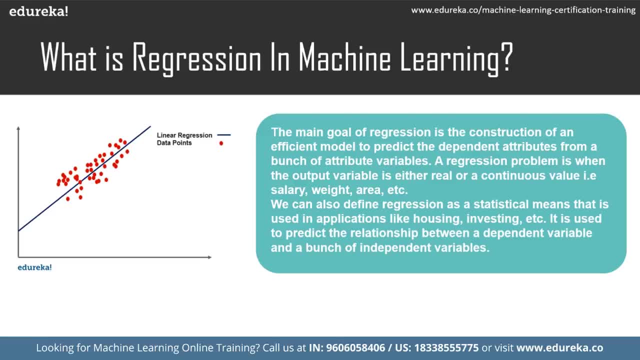 For example, let's say in the finance application or investing, we can actually predict the values of certain stock prices or you know those values depending on the independent variables like how many years it takes for a stock to you know actually mature, or how many days will it take to grow. 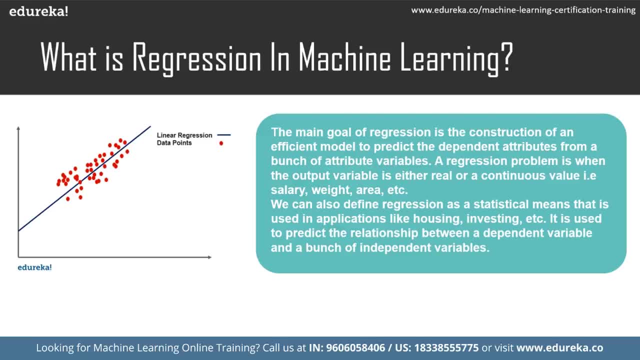 or those variables that you have in investing and depending upon that we can make a possible outcome or a possible prediction of how our stock is going to be invested- in a profit state or a loss state or all those things. or we can take another example like housing. we can take different parameters. 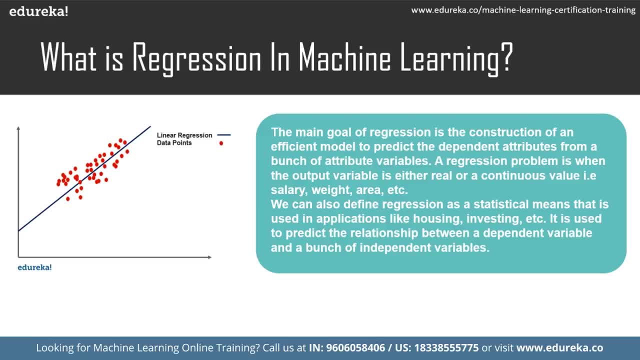 like number of years It's been there, how many people have used it or what is the area of the house. depending on all these factors, or how many rooms to the house have, we can get the price of a house. So this is basically what regression really is. 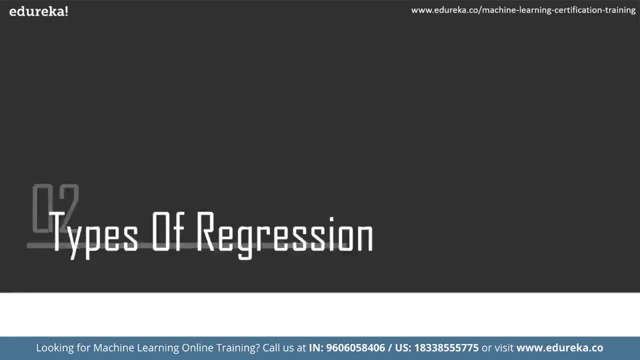 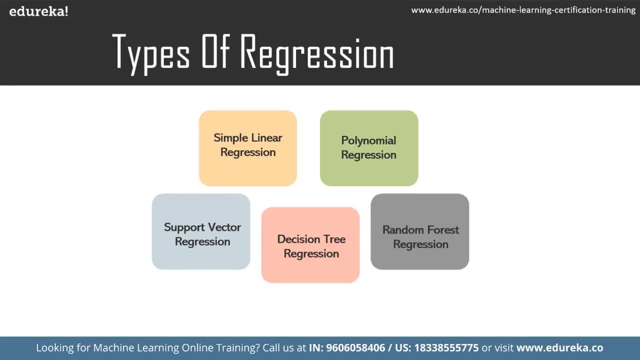 So let us take a look at various types of regression techniques that we have. We have simple linear regression, then we have polynomial regression, support vector regression, decision regression, We have random forest regression and we have logistic regression as well. That is also a type of regression that we have. 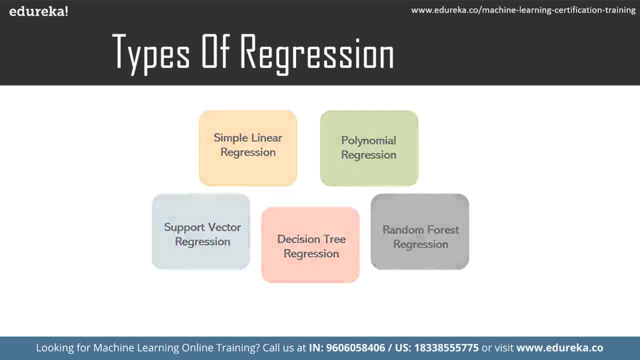 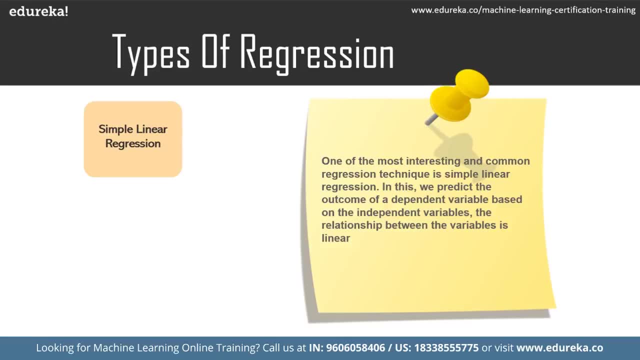 but for now we'll be focusing on simple linear regression. So let's talk about how or what exactly. simple linear regression first. So one of the most interesting and common regression techniques. This technique is simple linear regression and this way predict the outcome of a dependent variable, Y based. 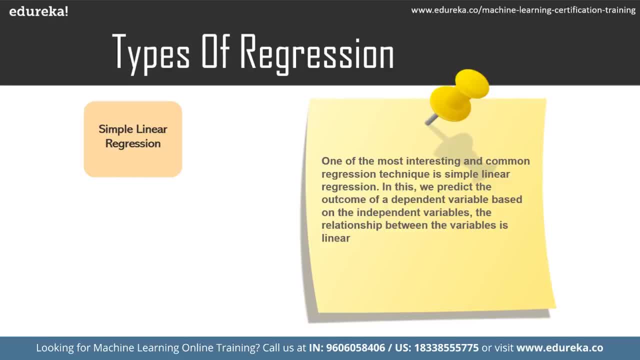 on the independent variables X. So the relationship between the variables is linear, Hence the word linear regression. then comes the polynomial regression. So in this regression technique we transform the original features into a polynomial feature of a given degree and then perform regression on it. 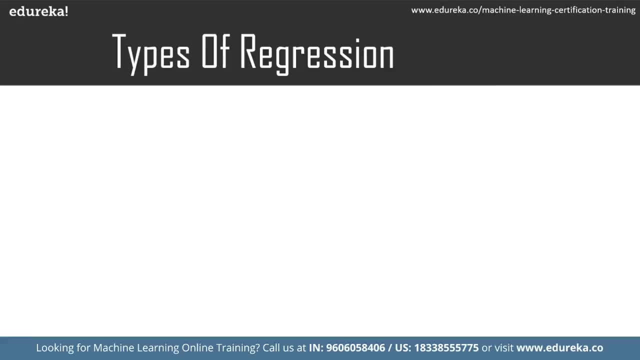 So this is basically polynomial regression. after this We have support vector machine regression, or we can also call it SVR. We identify a hyperplane with maximum margin, such that the maximum number of data points are within those margins. It is also quite similar to the support vector machine classification algorithm. 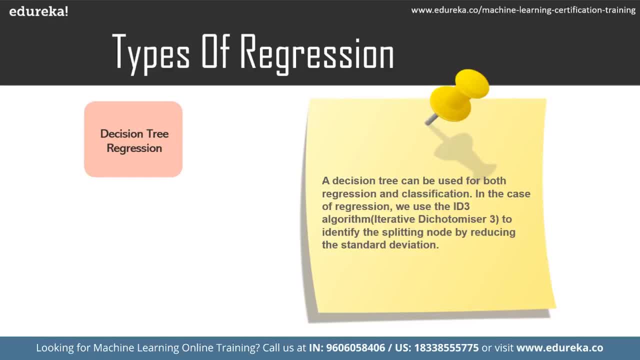 Then we have decision tree regression. a decision tree can be used for both regression and classification, But in this case of regression, we use the ID three algorithm, which is iterative dichotomizer three, to identify the splitting node by reducing the standard deviation after this: 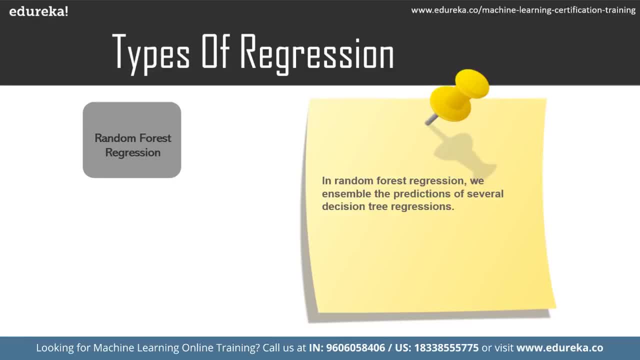 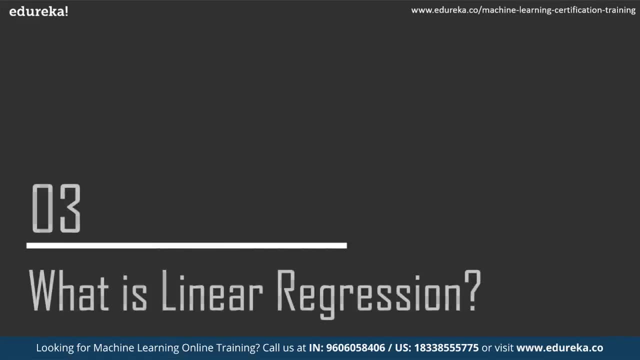 We have a random forest regression which is basically an ensemble of predictions of several decision tree regressions. So this is all about the types of regressions. for now, We are going to focus on simple linear regression. So let's take a look at what exactly is simple linear regression. 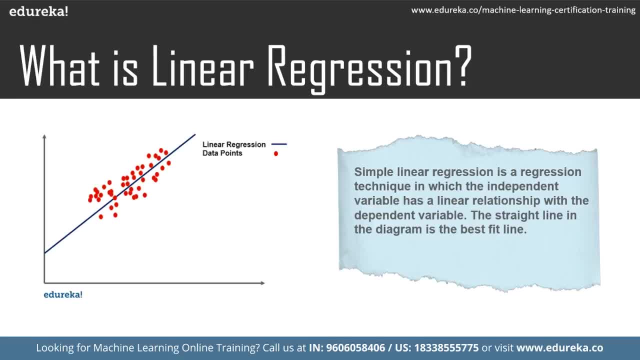 simple linear regression is a regression technique in which the independent variable has a linear relationship with the dependent variable. straight line in the diagram is the best fit line and the main goal of the simple linear regression is to consider the given data points and plot the best fit line. 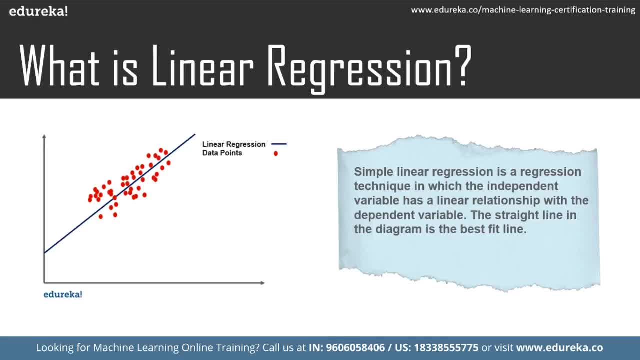 to fit the model in the best way possible. So if you talk about a real-life analogy to explain linear regression, we can take an example of a car resale value. So we have different parameters, you know when we are talking about a resale value of a car. 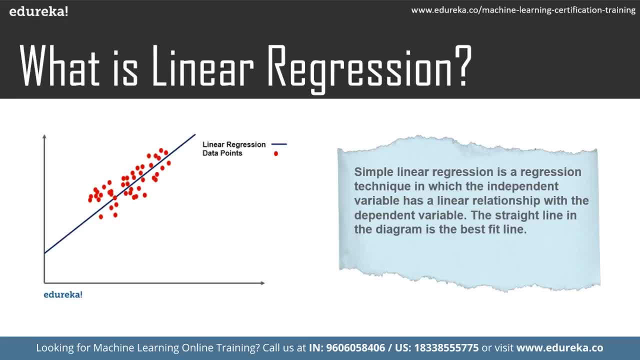 like how many years the car has been there in the market and how many kilometers it has been written, the kind of mileage the car gives, and then we have different parameters we can focus upon and all these independent variables somehow are linearly connected or interconnected to the price of the car. 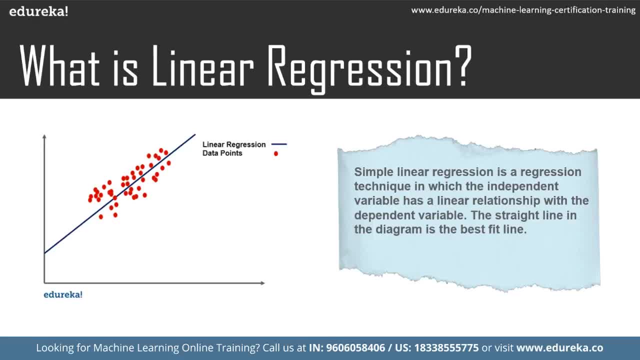 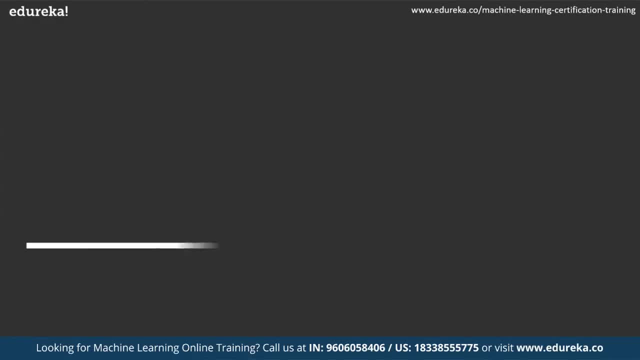 So that is one example to understand linear regression. We'll be doing that in the use case. I'll be telling you about how you can predict the price of car. now, talking about linear regression terminologies, There are a few terminologies They had you have to be thorough with to begin. 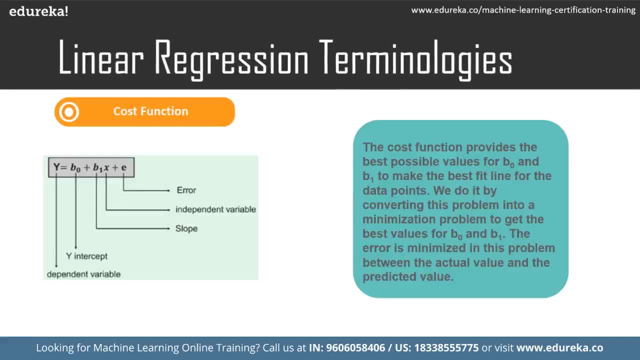 with linear regression. So first of all we have talked about cost function. So the best fit line can be based on the linear equation that is given here. So in this the dependent variable that is to be predicted is denoted by Y a line. 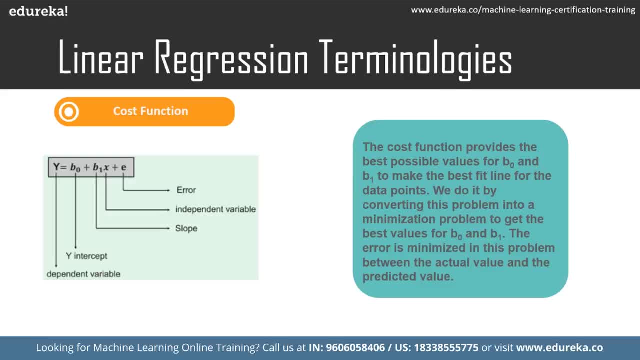 that touches the y-axis is denoted by the intercept B 0, the B 1 is the slope of the line and X represents the independent variables that determine the prediction of Y. the error in the resultant prediction is denoted by E. not talking about cost function, the cost function provides the best possible. 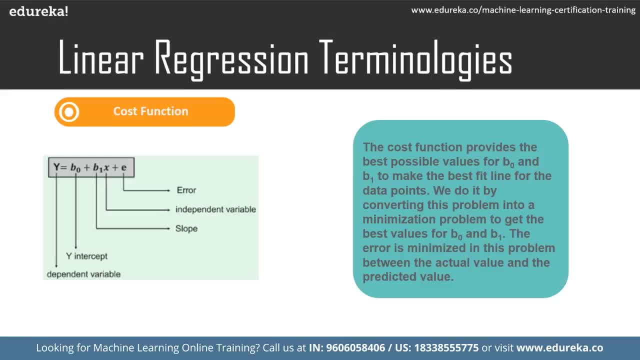 values for B 0 and B 1 to make the best fit line for the data points. We do this by converting this problem into a minimization problem to get the best values for B 0 and B 1. so with this the error is minimized in this problem. 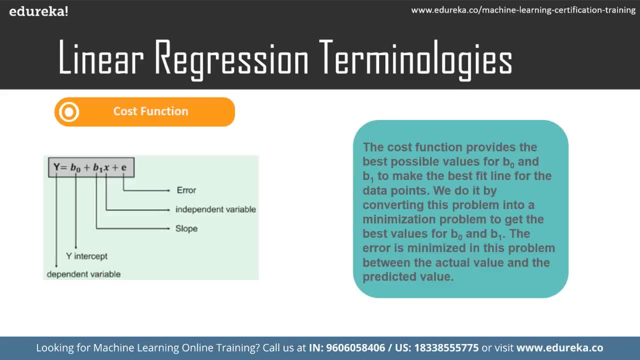 between the actual value and the predicted value and we choose the function to above to minimize. now we square the error difference and some the error over all the data points. the division between the total number of data points and the produced value provides the average square error. 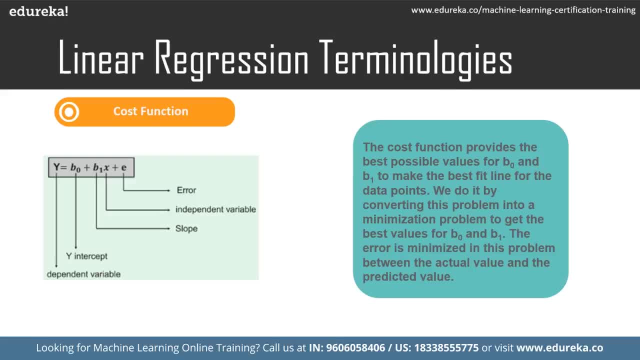 for all the data points. It is also known as mean squared error, and we can change the values of B 0 and B 1 so that the MSE, or the mean squared error value, is settled at the minimum. So this is one terminology that is cost function. 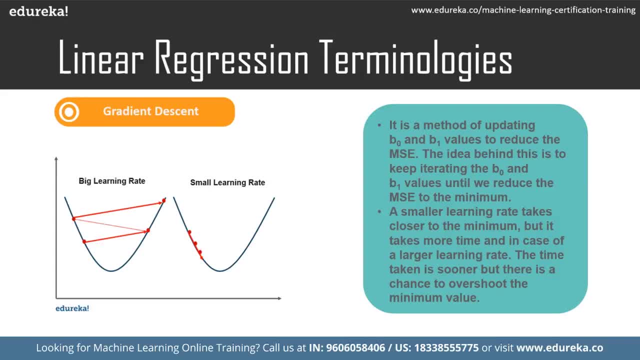 that we use in linear regression. Then we have the gradient descent. So the next important terminology to understand linear regression is gradient descent, of course, and it is a method of updating B 0 and B 1 value to reduce the MSE, which is the mean squared error. 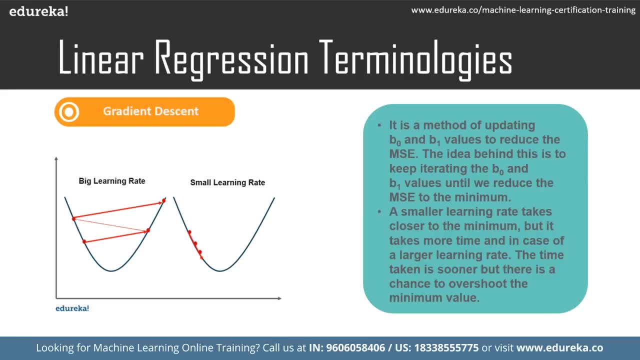 The idea behind this is to keep iterating the B 0 and B 1 values until we reduce the MSE to the minimum. now to update B 0 and B 1. We take the gradient from the cost function and to find these gradients We take partial derivatives with respect to B 0 and B 1. 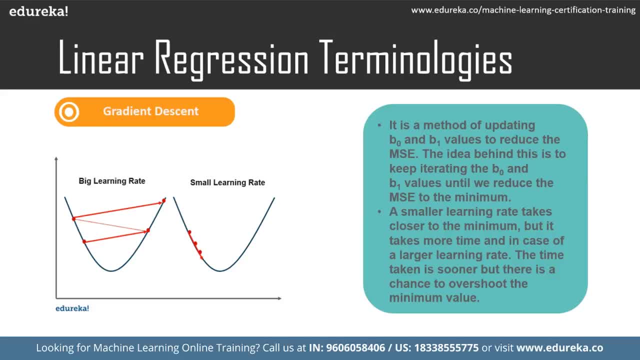 and these partial derivatives are the gradients and are used to update the values of B 0 and B 1.. I'm sure that this might be a little confusing for you guys If you are new to this- like gradient descent and cost function, but you don't have to worry about this. 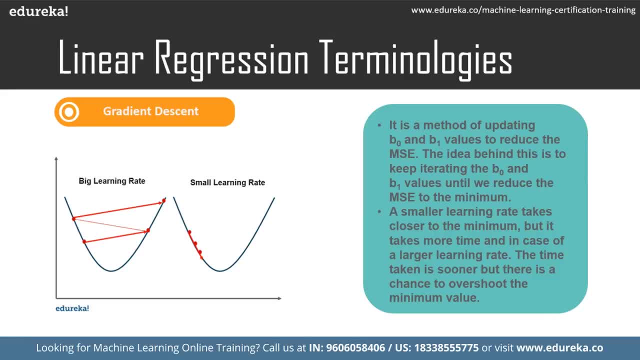 because in Python, when we're using a linear regression, we're going to be using the SK learn or the scikit-learn library, So you don't have to worry about this. You just have to integrate your model with the linear regression model that we have already over there. 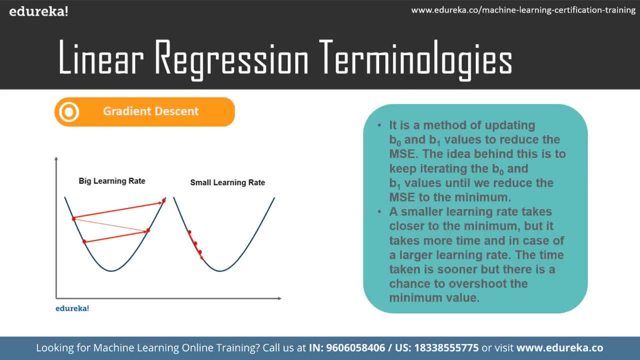 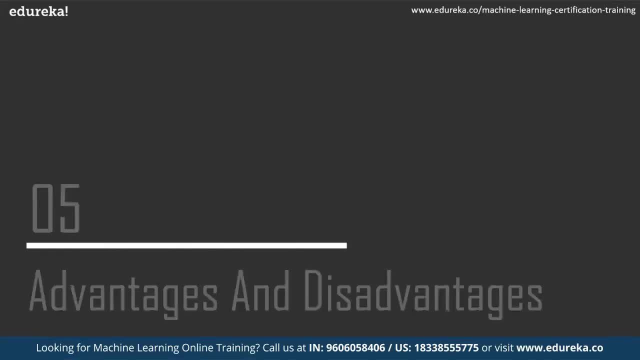 and you will be done with and when I'm implementing the linear regression model, you will see how easy it is to actually implement linear regression in Python. So after this, let's talk about a few advantages and disadvantages of linear regression. So, talking about the advantages first, linear regression. 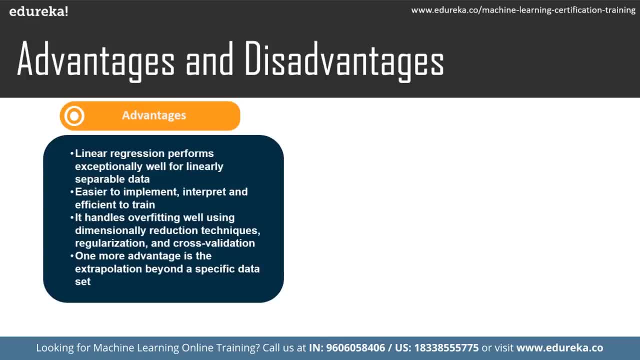 performs exceptionally well for linearly separable data and it is actually very easy to implement, interpret and very efficient to train as well. And even though the linear regression is prone to overfitting, it handles it pretty well using dimensionally reduction techniques, regularization and cross validation. and one more advantage is 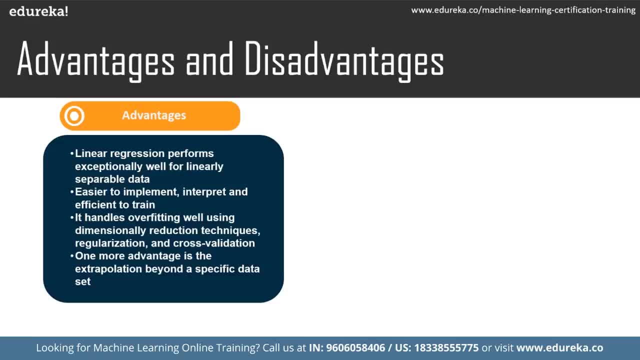 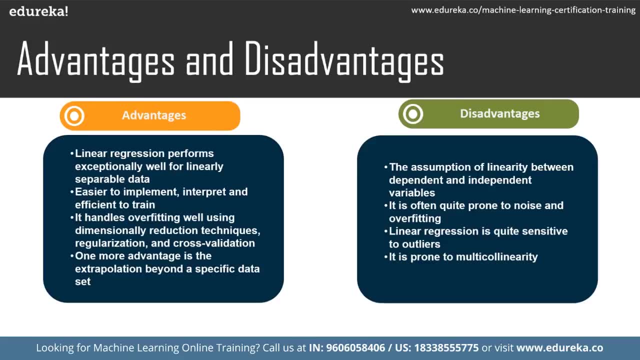 that the extrapolation beyond a specific data set. So these are all the advantages that we have with linear regression. Let's talk about a few disadvantages as well. So one of the most common disadvantage with linear regression is that it takes the assumption of linearity between dependent and independent variables. 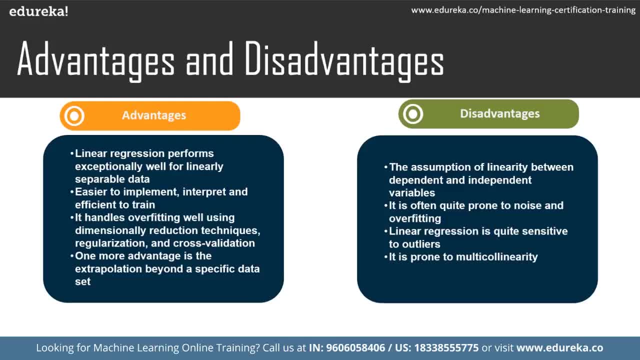 The next disadvantage is it is often very prone to noise and overfitting as well, which is not a very good sign for any model If you are doing regression or classification in machine learning. the next disadvantage is it is very, quite sensitive to outliers as well. 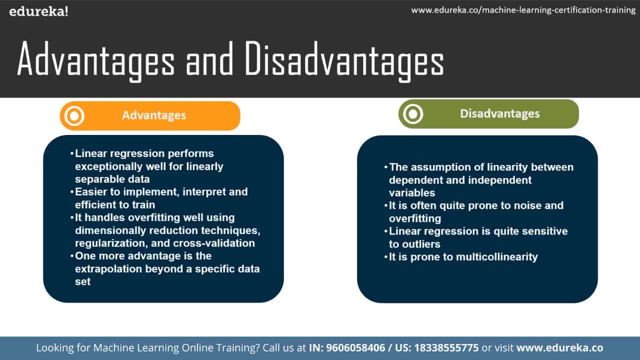 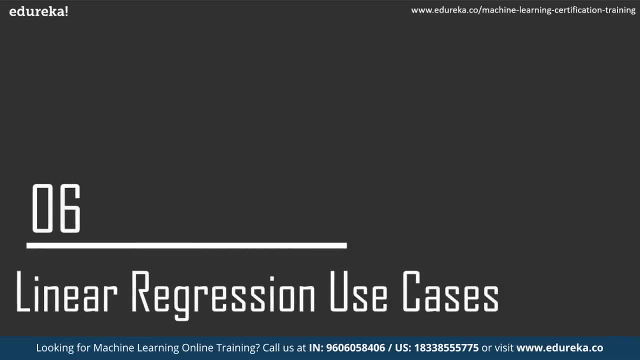 And the last one is that it is very prone to multicollinearity. So these are all the advantages and disadvantages of linear regression. Now let's also take a look at a few use cases that we can use linear regression for. so we can use it. 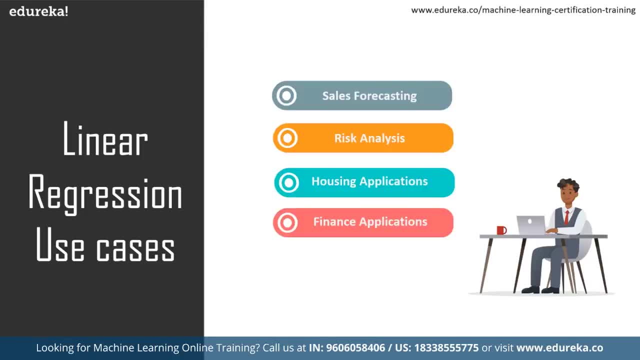 for sales forecasting, depending upon the features, like we can actually predict the price of a item or in sales. We can forecast the price or make assumptions over there like predictions. obviously then we can use it for risk analysis, for disease predictions, like we can take our disease data set. 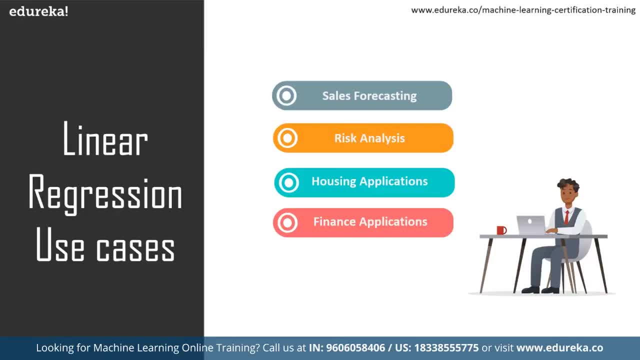 and, depending upon several features that are linearly connected with one: risk detection, We can use it for risk analysis as well. We can obviously use it for housing applications to predict the prices and other factors, like what are the different aspects that are going to be decisive in the price of a house? 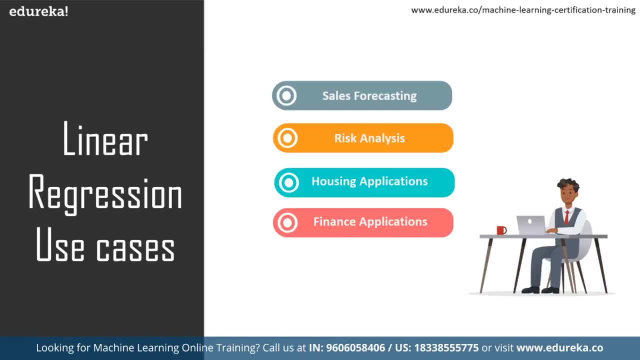 all those features using the linear regression. and then, of course, we can use it for finance applications to predict the stock prices, investment Evaluation, Etc. The basic idea behind linear regression is to find the relationship between the dependent and independent variables to get the best fitting line. 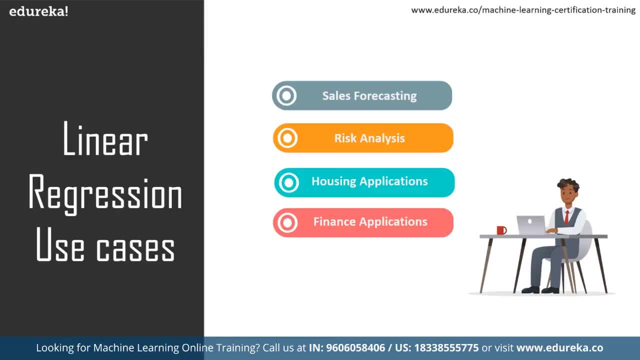 that would predict the outcome with the least error. so we can use linear regression in simple real life situations as well, like predicting the SAT scores with regard to the number of hours of study and other decisive factors that we can use it for, now that we are done with the use cases as well. 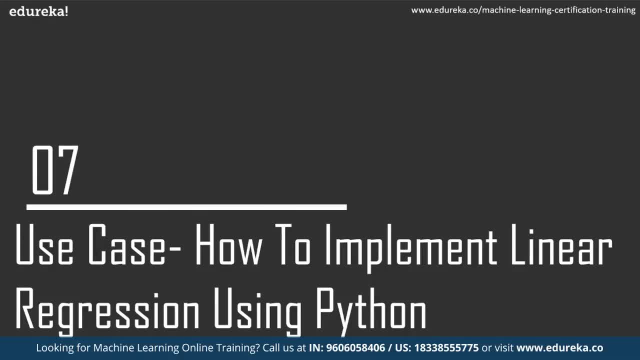 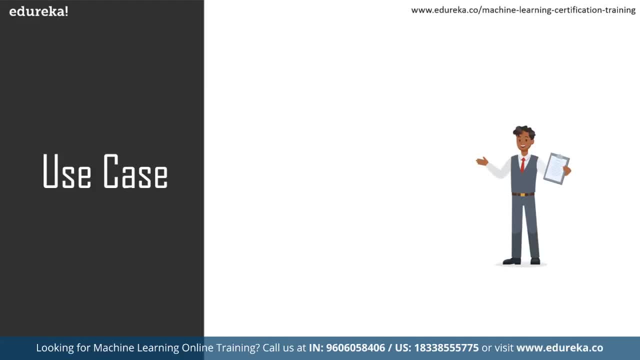 Let's take a look at specific use case that I'm going to show you in sklearn or scikit-learn library, and we're going to implement the linear regression model over there. So let me take you through the steps that are going to take place over there. 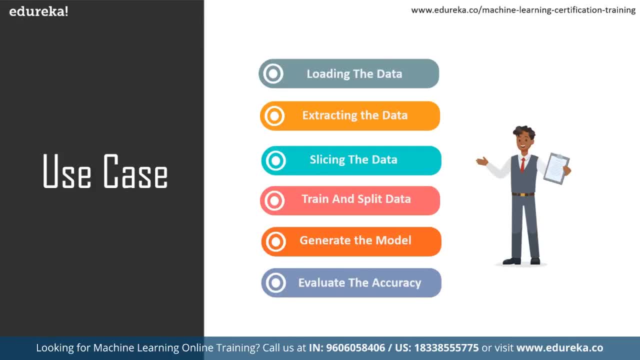 So first of all, we are going to load the data. after that We'll explore the data, So we'll take a look at how our data is, What are the different features and what are the data points that we have in the data set. 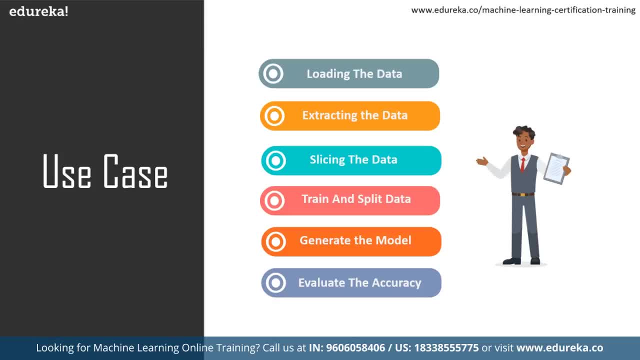 of that will slice the data according to our requirements and then we'll train and split the data using the fit and predict method that we have in scikit-learn and then we generate the model from scikit-learn and after we are done making the model, 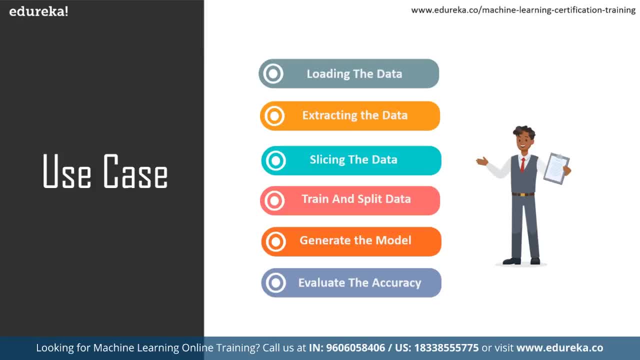 we'll evaluate the accuracy. So let's take it up to PyCharm guys. I'll show you a very simple example. First of all, with the diabetes data set that we have in scikit-learn, we can simply import it from the data sets module that we have in scikit-learn. 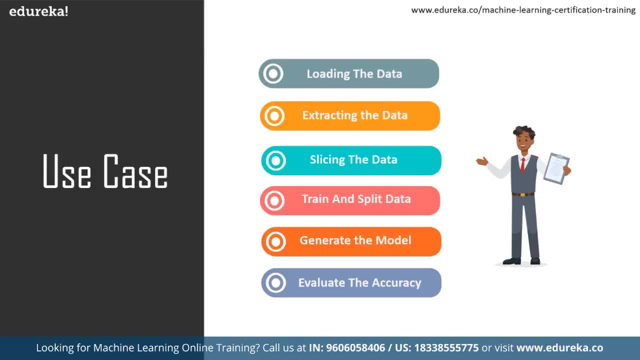 and after this simple example, I'm going to show you a custom data set, that is a car resale value, and we're going to put it some prices for car resale values. So, without wasting any more time, let's take it up to PyCharm. 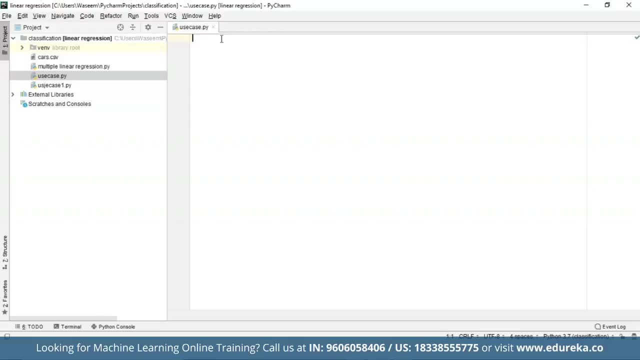 So now that we are in PyCharm, guys will try to implement linear regression using simple data set that we have in a skill on library. So first of all we'll have to import basic libraries like matplotlib. I'll make it a little bigger for visibility. 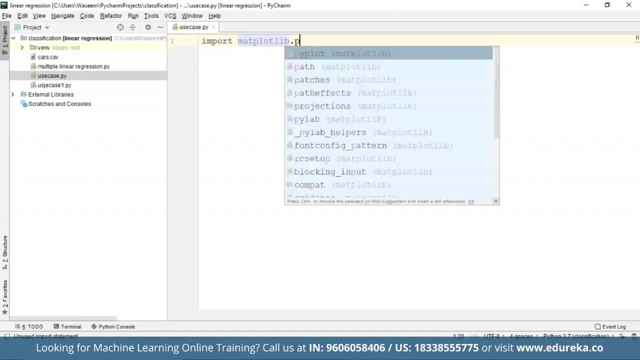 So first I'll import matplotlib Dot by plot, as let's say PLT, and after that I'll import numpy as NP, So from a skill, and we'll have to import data sets because we are going to use the data set from the data sets module. 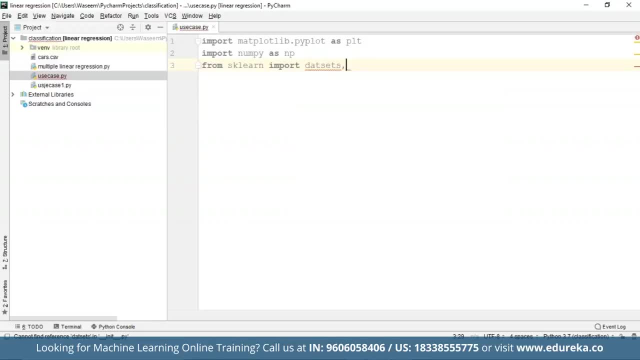 And we are going to import linear model as well, for linear regression can made a mistake over here And again, we have to import metrics for accuracy evaluation and we'll be importing mean squared error. So these are all the libraries that I'm going to use. 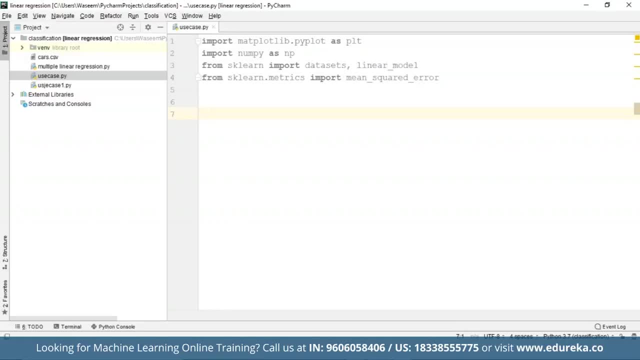 to show you how you can implement linear regression. But before that, don't make a mistake of using these libraries just as it is, because I have already. I already installed all these libraries, So for that you can just go to the project interpreter that you'll find in the settings. 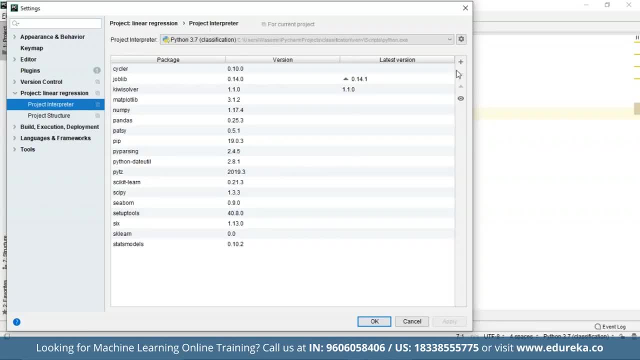 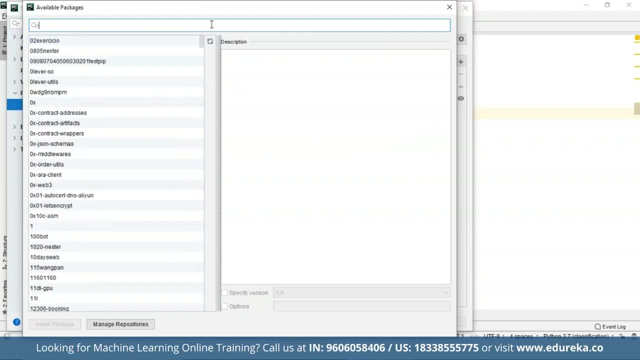 and over here you can just install all the packages that you need. So this is the add button. there You can add all the libraries that you need. So for sklearn you can just type sklearn and install that library. I'm not doing that again, because I've already done it. 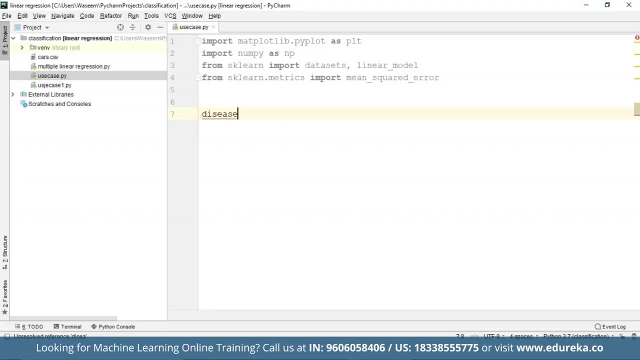 So after this, first thing that you have to do is import your data set. So for that, I'm taking a variable disease and datasets dot, load Load data sets, or I'm just going to load diabetes, because that's the data set that we are going to use in this. 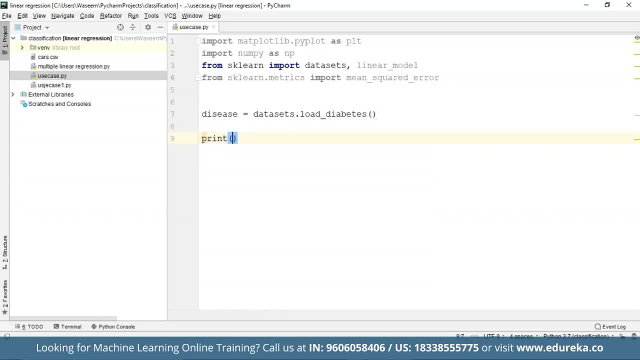 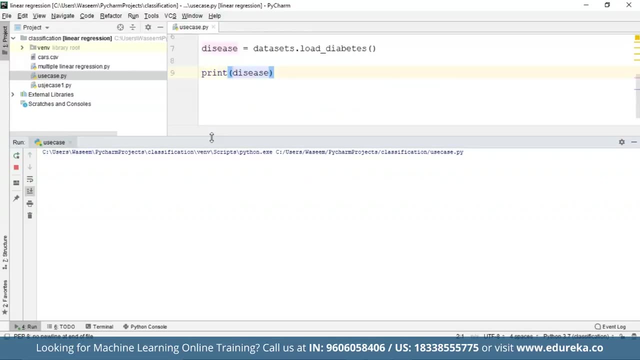 and let's just see what all we have in the data set that we have over here. So I'm just going to print this to know what all we are dealing with right now. It's going to take a while. So this is our data set, guys. 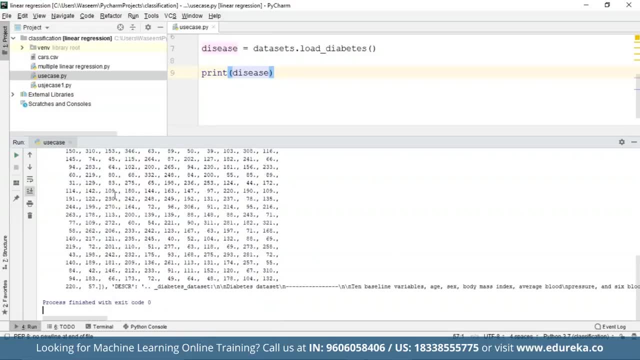 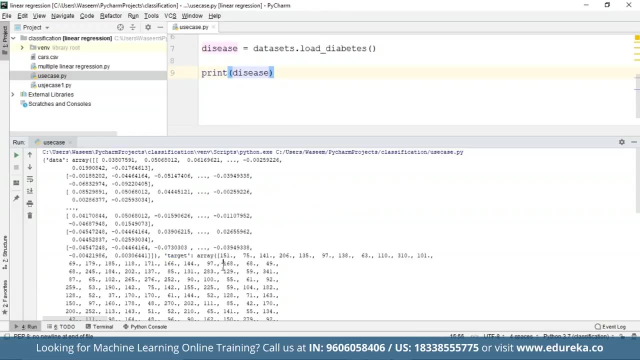 We already have a data over here. I'm sure we will be having a target. We have description over here, So this is our data set. guys, We have a target also. So this is a very sliced up data which is actually pretty good for our use right now. 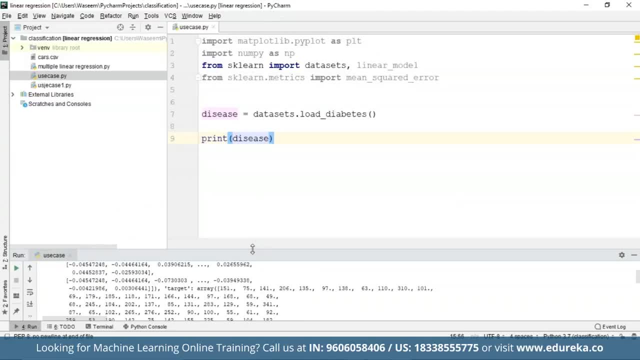 because I'm showing you a simple implementation of linear regression. So this is going to be very easy. So what I'll do is I'll comment this line, because we don't need this right now, And after this I'll just take one more variable. 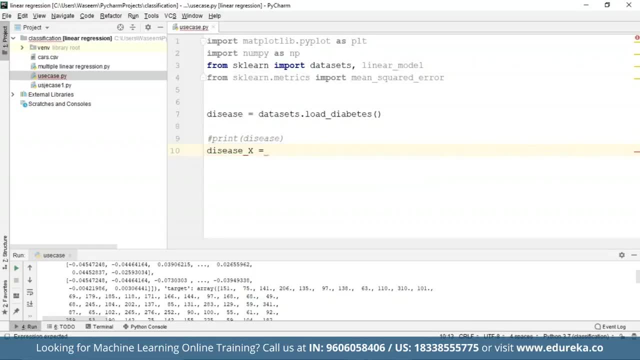 Let's just say disease X, and inside this I am going to take disease dot data. Now, after this, I'm going to split my data into train and test. so what I'll do is I'll just write disease X out of this. I'll write train. 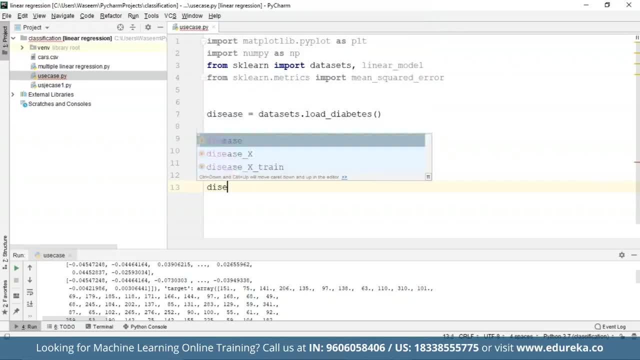 And let me take another variable, that is the X test, And we'll have to take this same variable for Y as well, because we need two variables. So I'll take it as Y, Train and disease. Why test now? inside this? I'll have to split my data into training and testing data. 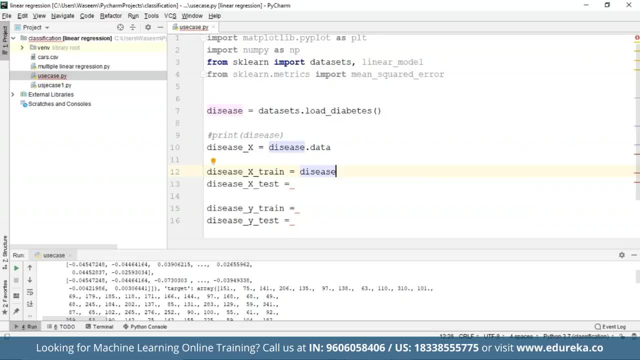 So I'll use the disease over here, or we can just call it data, also disease X, and I'm going to split the data from the starting until minus 30. So I'll leave the last 30 data entries inside the data set which I'm going to use in the training set. 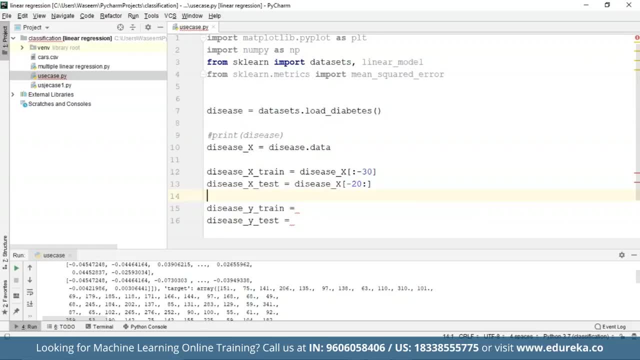 So I'll use for the training set the minus 20 that is, from the last, the 20 entries that we have over here, and similarly, in the same thing We are going to do for the white train and y test as well. So, yeah, I'll just write why. so, before doing this, 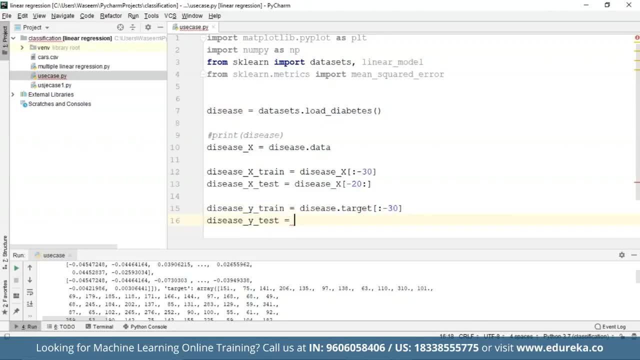 I'm just going to me as Target, because we're using the target variable over here. This is dot Target again, And in this I am going to use the last 20 entries. So we have successfully split our data. Now what happens is after splitting. 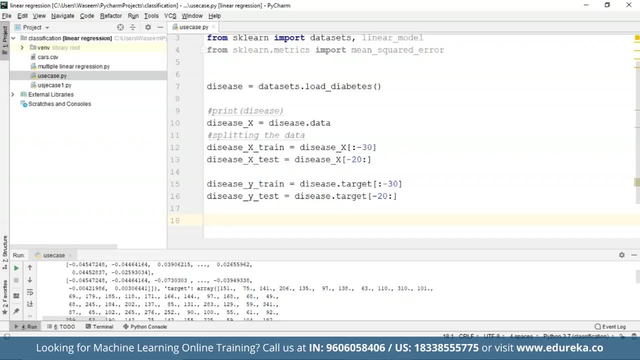 Your data. you have to generate your model for that. I'm just going to take one variable. So I'm just going to take it as reg or regression. We can call it as regression as well. So I'm going to use linear model. 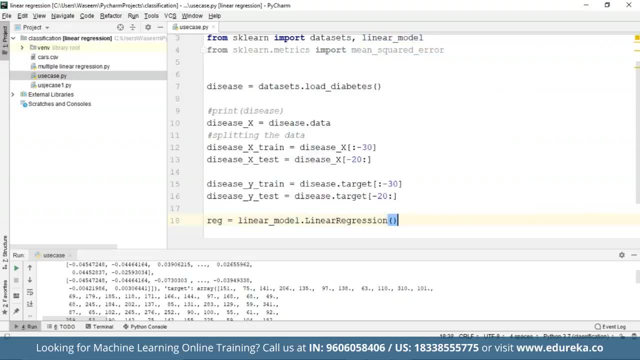 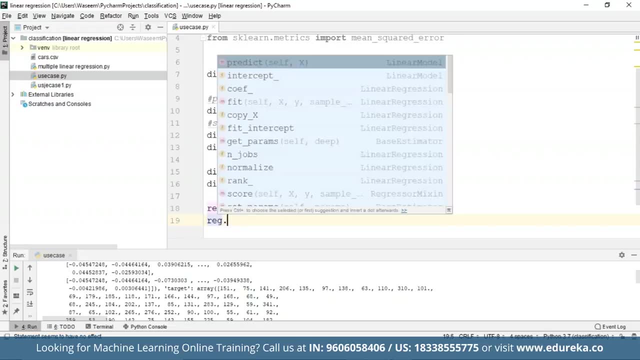 And I'm going to call linear regression. So this is how you can generate your model. So after this you have to fit your training data inside the model using the fit function. So I'll use fit over here and to fit the data I'm going to use disease X train. that has the data variables. 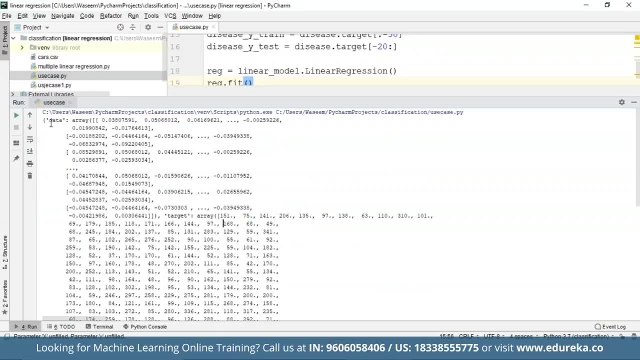 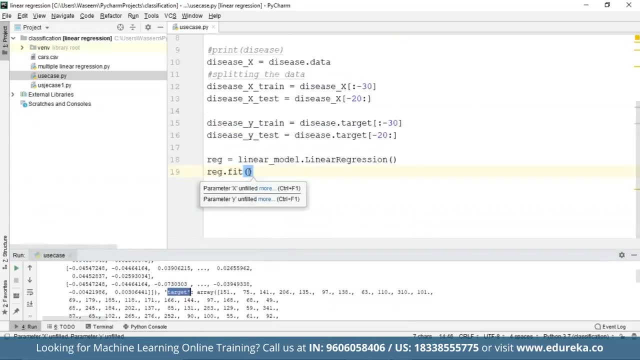 all those values that we have over here. That is this one. this array is going to be in the training one and we're going to use the target one for the disease Y, So I'll just do that. This is X train and disease Y train as well. 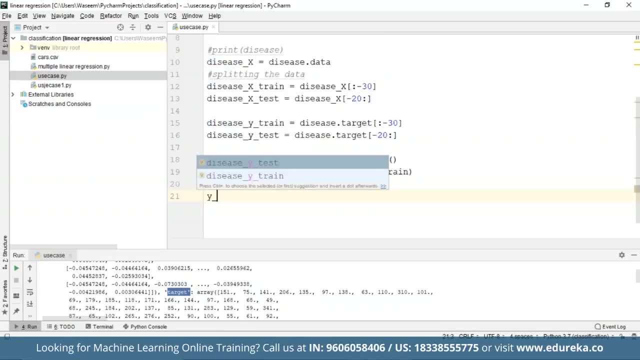 So we're done. after this, I have to make a prediction variable as well. I'll make it as my predict and inside this I am going to use the predict function. so for this we are going to use a disease X test, because this is what we are testing right now. 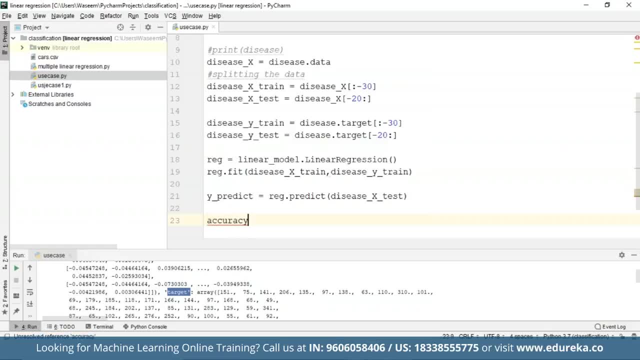 So our model is actually done, guys, I'll just write some code for checking the accuracy as well, So I'll use the mean squared error over here and inside this I'll pass disease Y Test and the y predict that we are going to get. 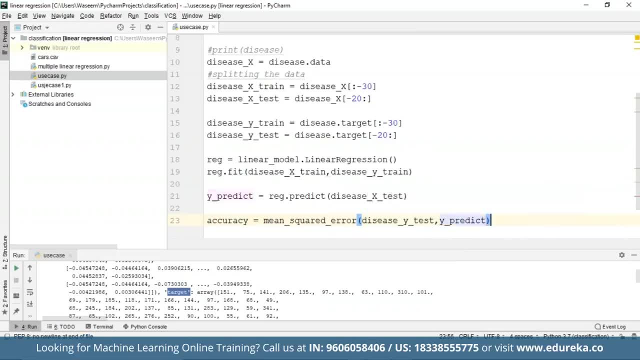 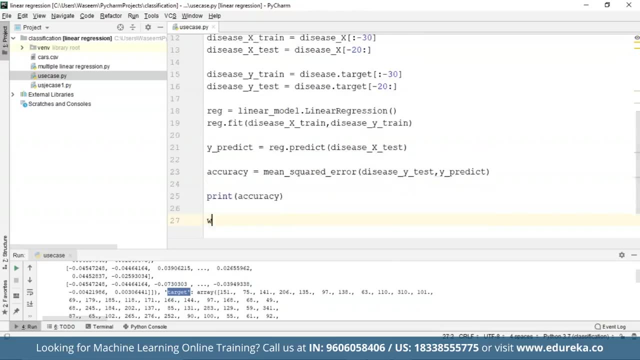 after the prediction. So we're almost done. after this, I'll print the accuracy as well, Whatever we will get, and let's just print the weights and the coefficients as well. So, as you say, weights is equal to reg dot, So you have a function for this as well. 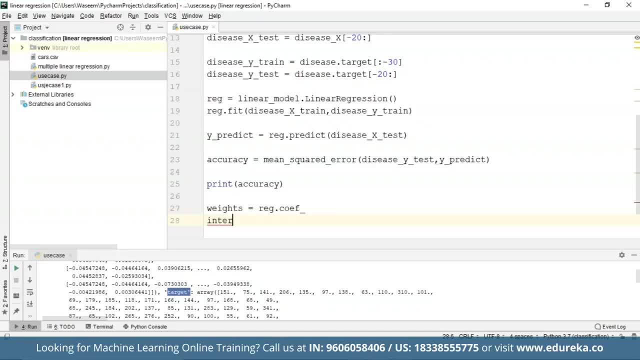 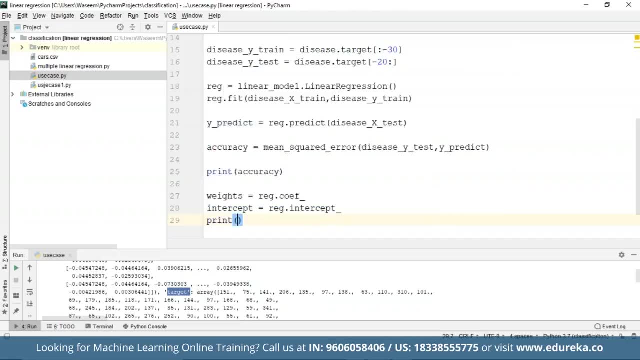 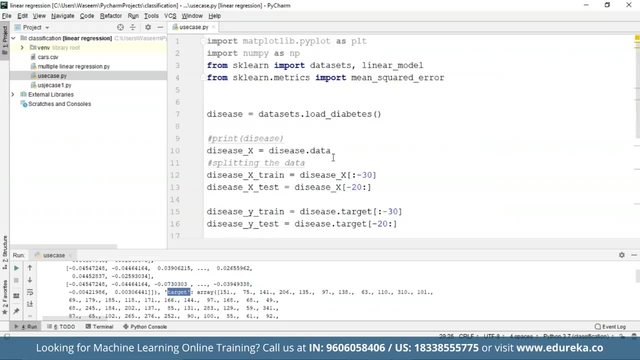 to calculate the coefficient, that is, the weights, and intercept as well. So I'll name it as intercept and RG dot intercept. We'll print these as well. Wait and intercept. so we are. model is done, guys. So I successfully used all these libraries. we have. load the data set. 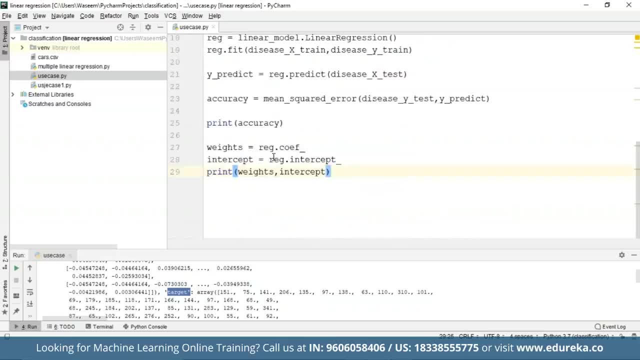 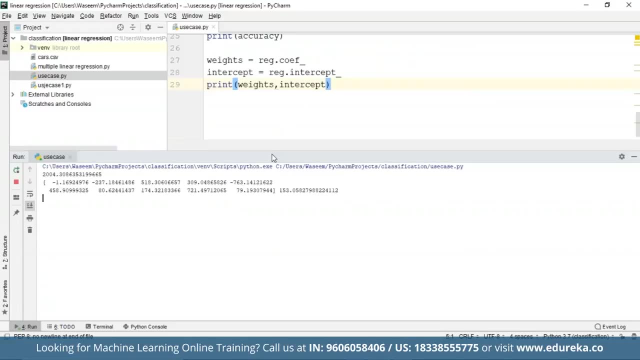 and after that we have generated the model by splitting the data and everything. So I'll just run this code and see what the output is. Okay, so we have the accuracy. that is a mean square error. That is 2004. and then we have the intercept and the weights as well. 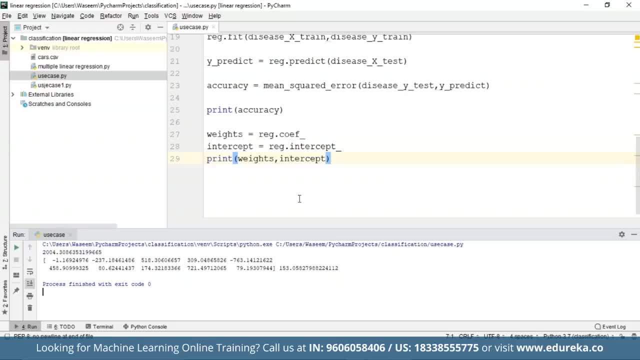 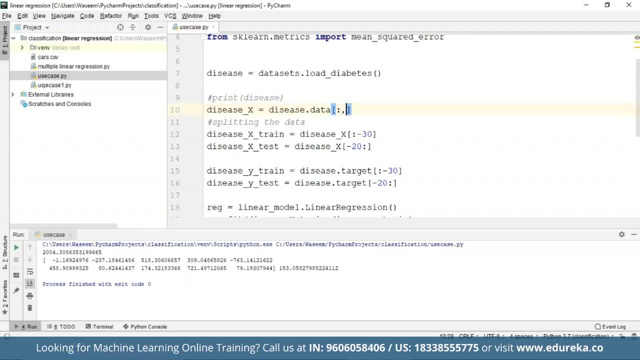 So this might sound a bit confusing for you guys. So I'll just add a few things over here to make you understand this better. So what I'll do is I will make a few changes over here, So I'll just write it like: NP dot- new axis, lighted as two over here. 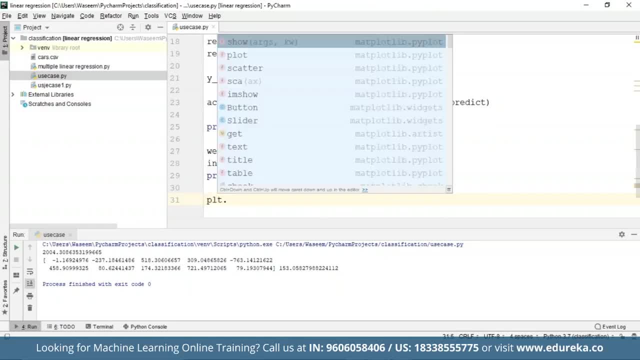 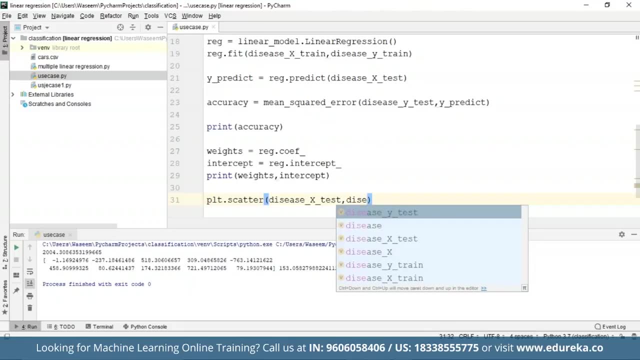 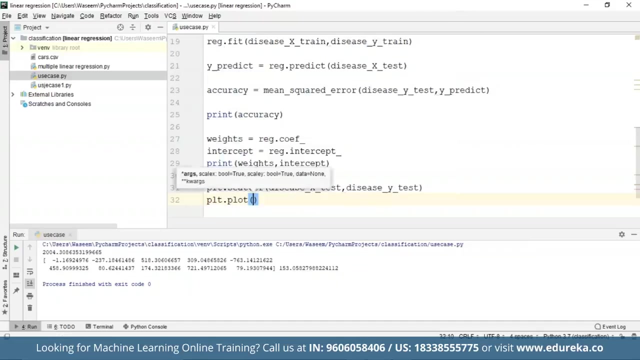 and we'll plot the graph also. So for that I'll just write plot scatter. inside this I'll use disease dot X test disease, not white test. PLT dot plot for the line, and inside this I'm going to use disease X test and y predict. 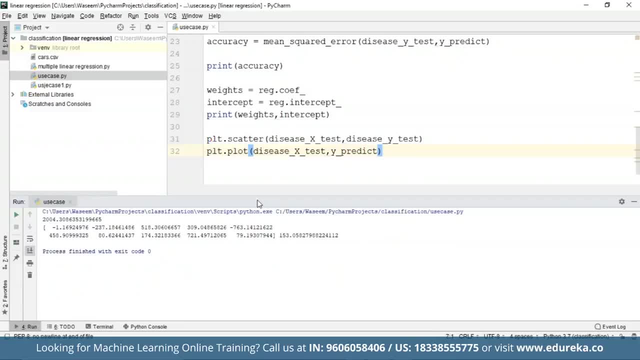 So now, when I run my code, you will be able to see the graph which will have the data entries, And you'll be able to see the graph which has the data points, and there will be an intercept as well, with a line plotted which is the best fit line over here. 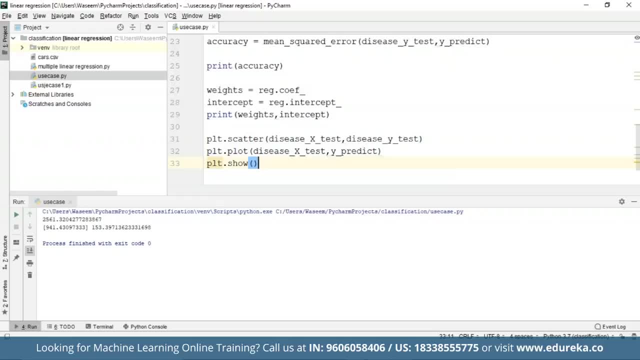 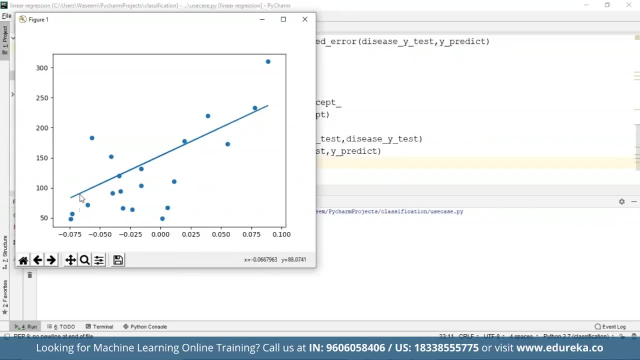 Okay, we have not written PLT dot show. That's why we're not getting the graph now. It should be fine And we'll be able to see the graph as well. So this is our best fit line, guys. So we have successfully implemented linear regression. 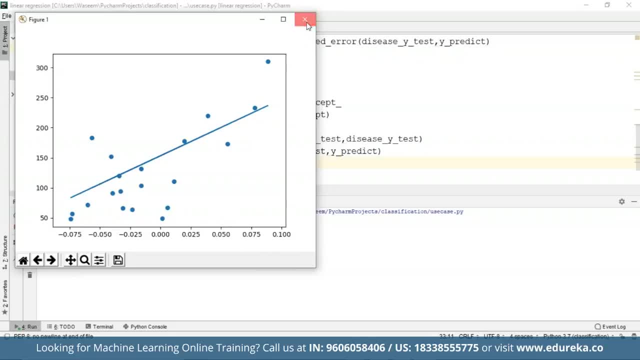 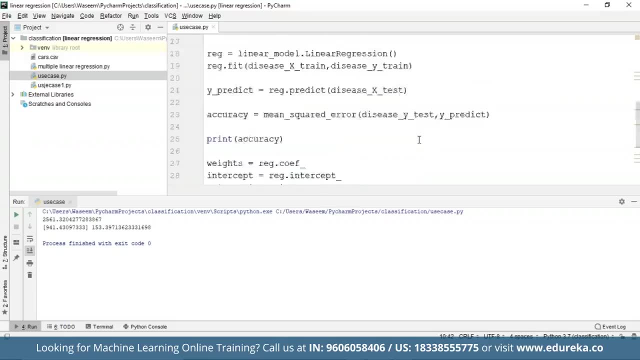 using python for this disease data set. But to do this I had to segregate this data All separately and if you implemented using all the columns that you have in over here in the data, it's not going to be fine. I mean, it's going to throw you an error. 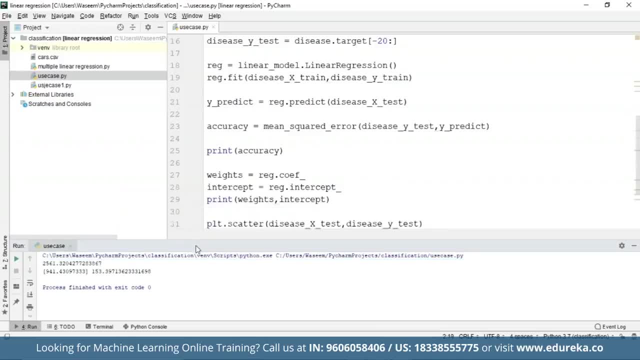 and with not show you a best fit line. So now that we are done with this one, I'll show you one more use case. inside We are going to use the custom data set, which has the car resale value. So let's get it done. 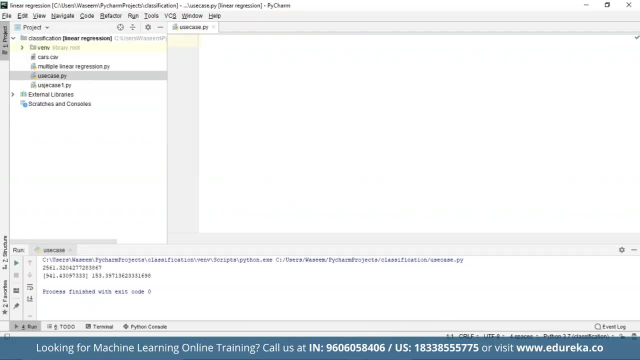 So I just remove all this. So first of all, I will import, as you can see over here in the directory, guys, you can already see this: cars X- CSV. This is my custom data set that I'm going to use inside this one. 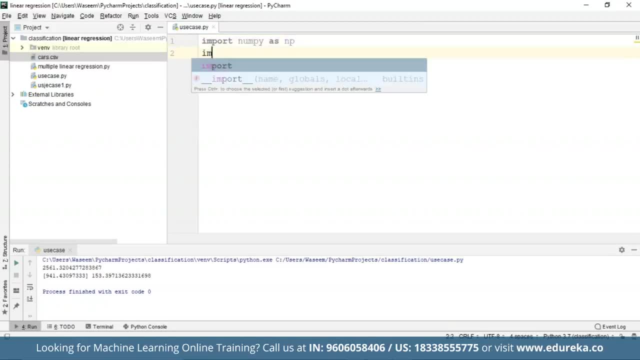 So I'll just import numpy as NP, Import pandas, because we are using our custom data set. I'm going to have to use pandas to import or to actually load the CSV file that I have over there, and after this I'll use map, dot, lip, dot pi plot as PLT. 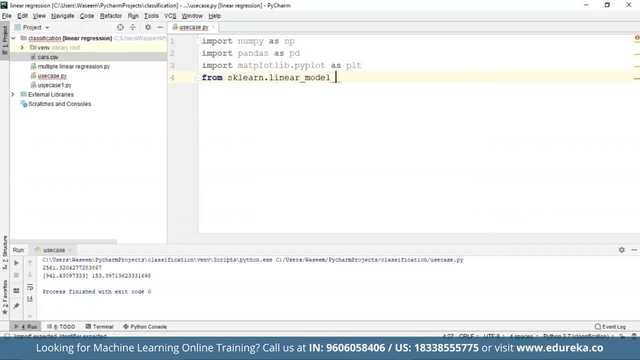 and from a scale on linear model. We are going to use linear regression And after this I'll just import a scale on, not metrics, and import the r2 score, or we're not going to use that, So I'll just remove this one for now. 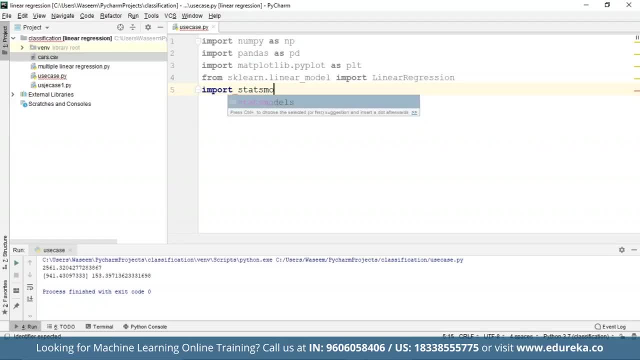 and we'll use import stats model. We leave this one for later as well. So first of all I have to load the data. So I'm naming it as cars. So for this I'll just write PD, rotary, CSV. And if you don't know how you can import the CSV files, 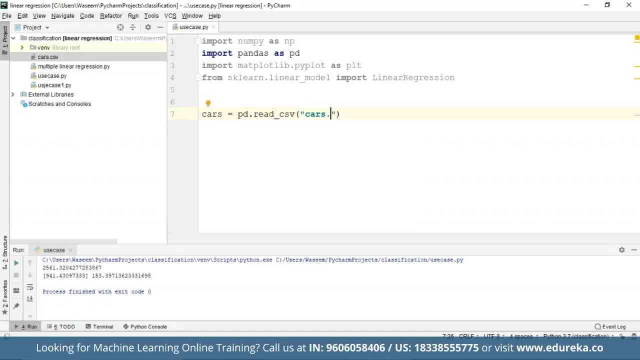 the custom made CSV files. inside your program you can check out other tutorials on the end You record. so we have a tutorial in detail how you can do CSV files. So first of all let me just get a quick exploration of the data, what we have over here. 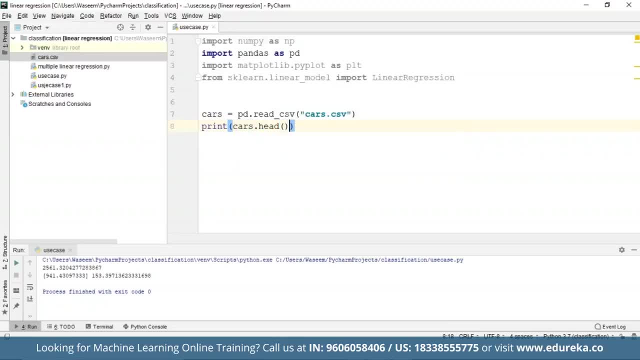 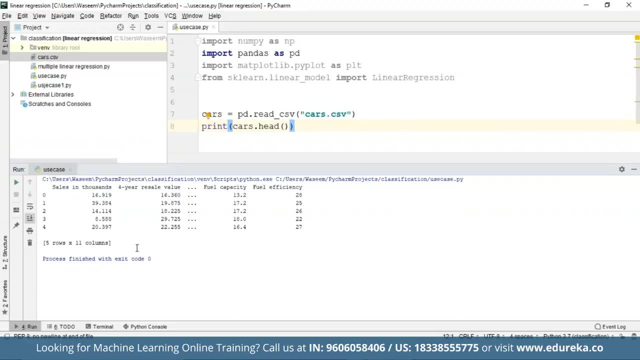 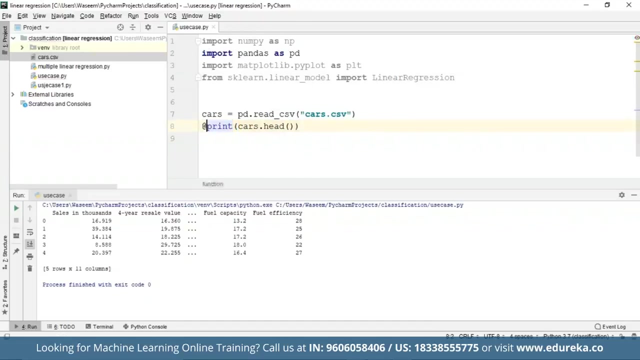 So I'll just write the print statement. I'll get the head. So this is what my data set looks like. guys, It's loading still. so we have all these values and to get the better picture over here, I will try to print. 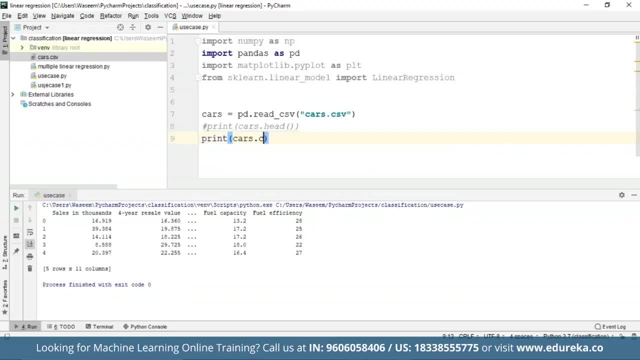 The columns as well. So I just write cars or columns, So it will give me the name of all the columns that I have in this data set. Okay, so we have all these values, sales in thousands. We have a four-year resale value. 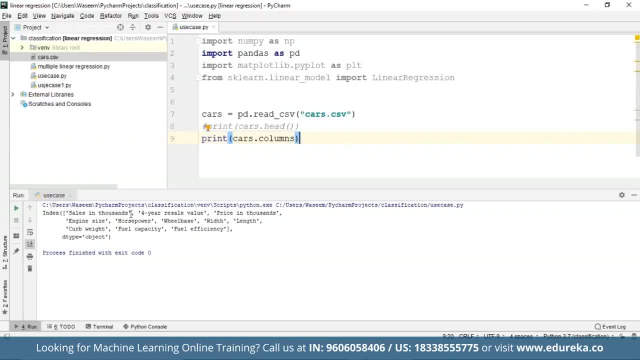 then we have price in thousands, and we have engine size, horsepower, V, base, width, length, Then we have cup weight, We have fuel capacity, fuel efficiency as well. Okay, so this is what our data looks like, guys, So let me just plot a graph, first of all. 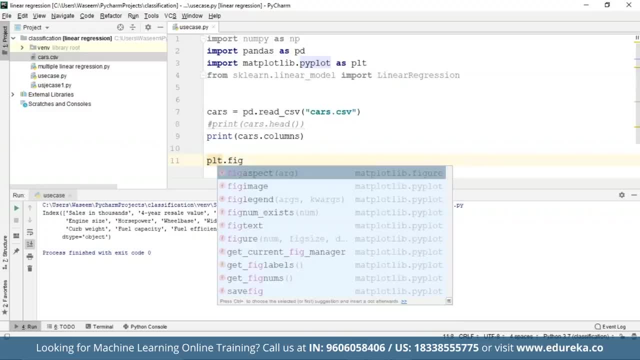 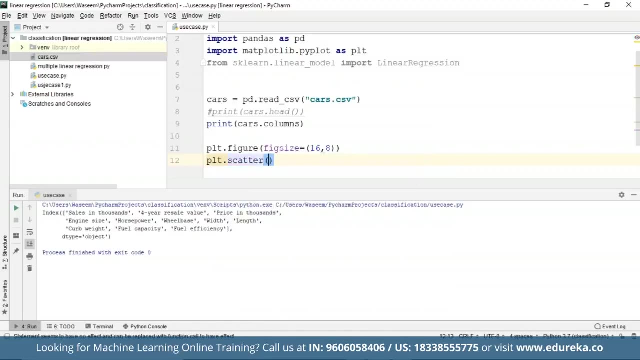 So I'll just write PLT And you're going to use the figure size, For figure size is equal to, let's just say, 16 by 8. and after this I will use a scatter plot And inside this I'm going to give a few values. 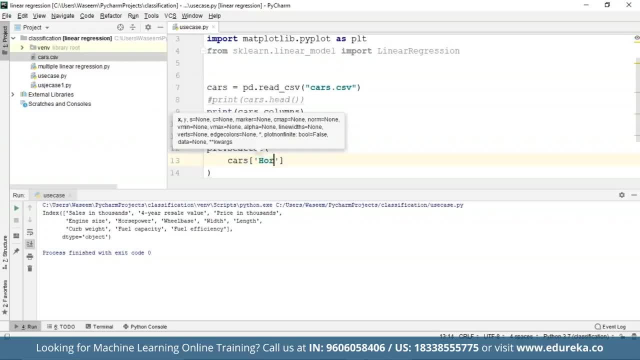 So I'm going to use cars. So first of all, I want to check the relationship between a horsepower and then I'll check what is the relation between a horsepower and the price of the car, which is in thousands, of course, And let's just get it as black. 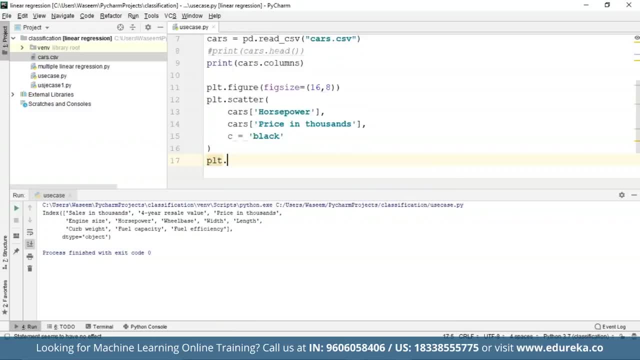 Yes, and let's just put a few labels as well. So X label is going to be, let's say, horsepower, And we will write the Y label as let's just say price, And let's just plot this graph for now We- I'll put it over here only now, when I run this- 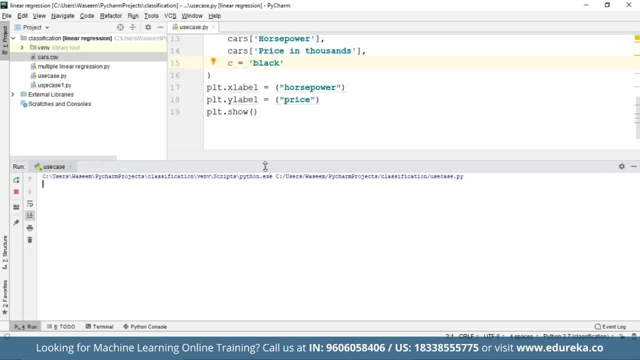 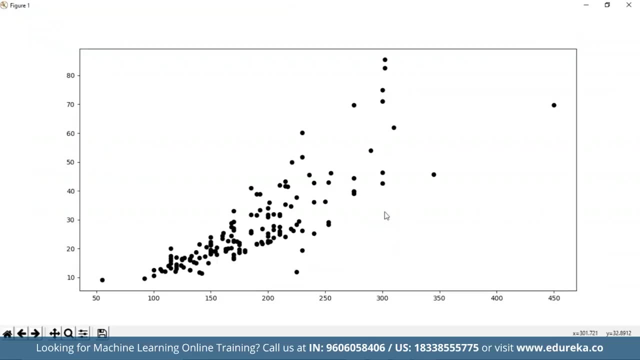 let's see what I'm getting over here. So I'm getting a graph like this So you can see all the data points and as we go further, the values are actually increasing. if you're not getting the Y labels over here somehow, I think there's some problem. 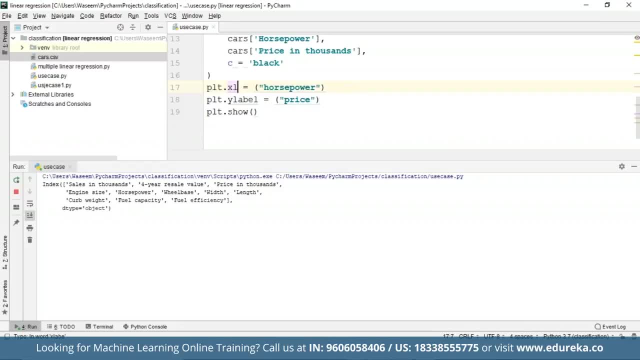 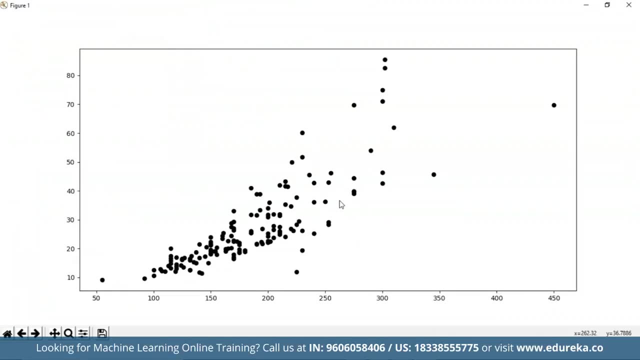 Just check it out. Okay, we leave it for now and let's check the image of over here. So on the x-axis we have the horsepower, which is going until 450. So a car with the horsepower 450 is ranging around 70,000. That is the price and that's going to be in dollars, guys, and all these values, like a 150 horsepower car, It's going to be around 20,000 bucks and a simple 50 horsepower car is going to be around 10,000 bucks. 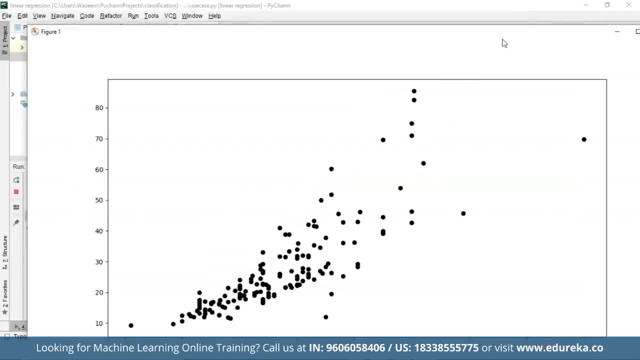 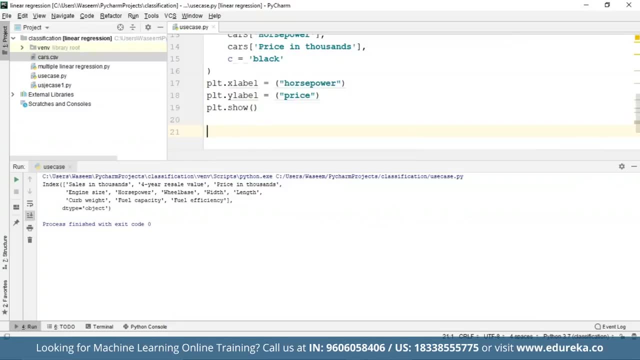 So this is our data, guys, I think it's pretty evident that we have a relation between a horsepower and the price of the car that we are actually looking at right now, So we'll build a model around this for now. So I'll take one variable. 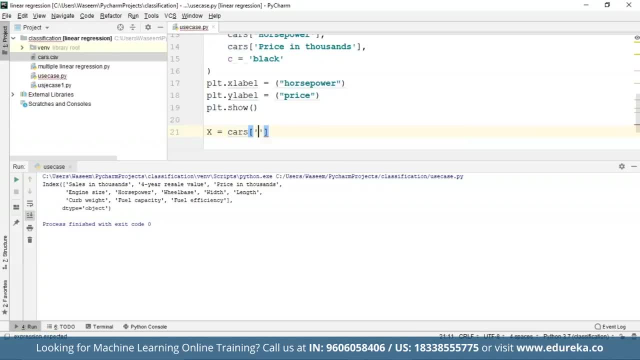 Let's just say X, and inside this I'm going to put cars, horsepower, because we are going to take horsepower as our independent variable. and all these values, I'm going to reshape them into minus 1 and 1.. I'm going to take one more independent variable. 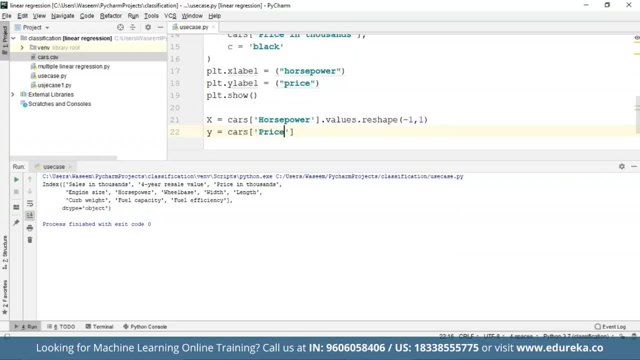 Why that's going to be my price in thousands guys. I'm going to do the reshaping again. Is this basically to avoid the errors, guys? reshaping that I'm doing over here and I'll just generate my model right now, So I'll use linear regression. 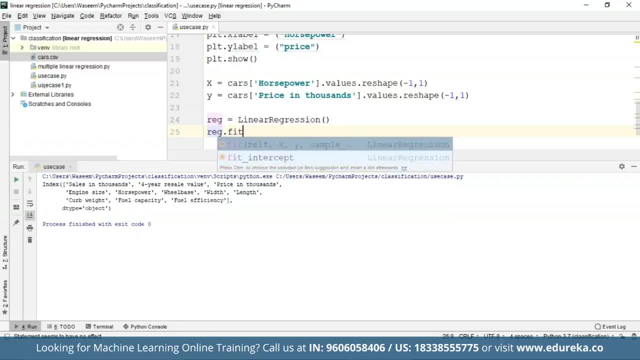 And after this I'll try to fit my x and y over here using the fit method. So just write x and y. Now I'm going to print the coefficient using the coefficient function that I've shown you before. I'm going to take the values as 0 and 0.. 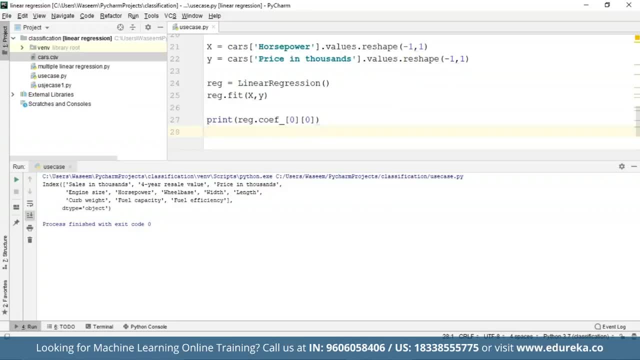 Again for the same thing. I want to intercept as well. changed of coefficient. I'll write as intercept and I'll remove this one After this. let's make one variable, Let's just say predictions- that's going to store the predicted value and we're going to use the predict function over here. 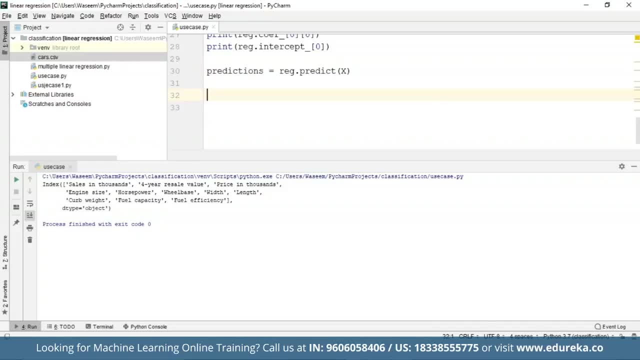 So I'm just going to put X over here in the predict function and let's just plot a graph again. So right, figure, figure size again. Let's just take 16 by 8.. We'll use the scatter plot again. We just write it again. 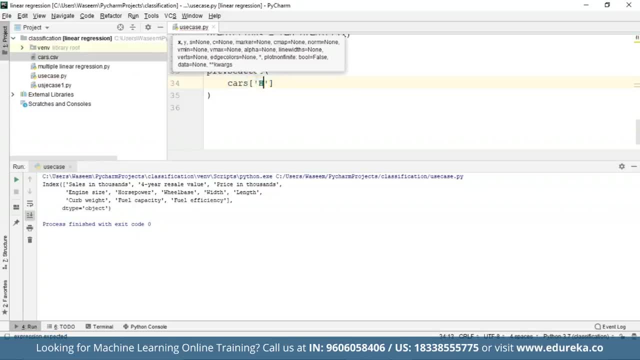 First of all, we have cars and horsepower. Then we have cars: Prize In thousands. After this, I'm just going to write: C is equal to black. Now we have one more plot for the line, So I'm going to use PLT dot plot inside this. 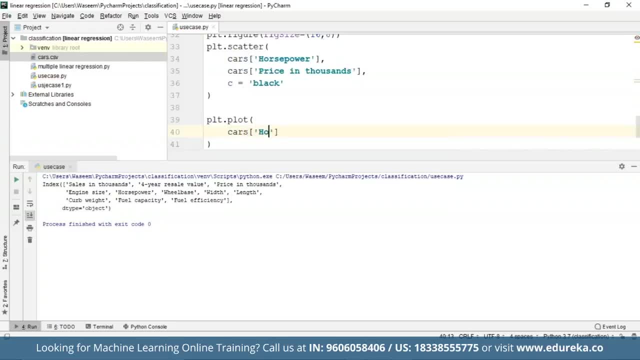 We'll have cars, horsepower. We'll use the predictions as well, And let's just make it blue. We'll put the label again, So the X label is going to be The horsepower And the Y label is going to be Prices. 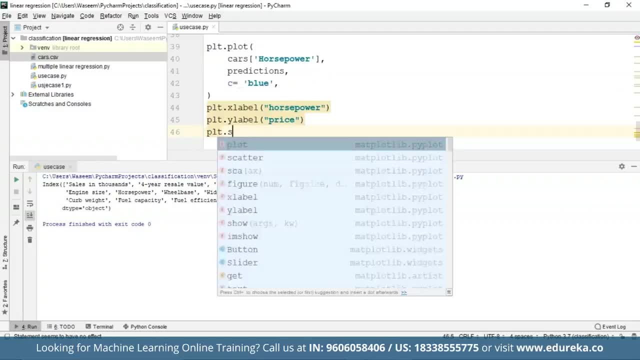 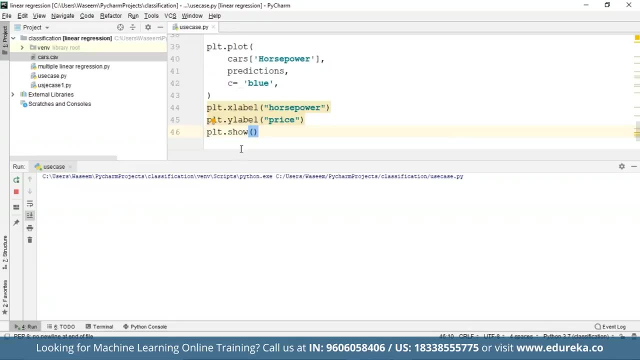 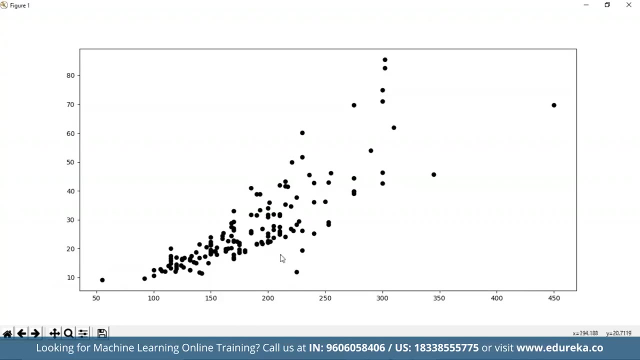 I'll just price. I'll write: PLT dot show. Now, when I run this, I should be getting a. okay, We'll get the first plot before getting the second blood. So we have a plot like this. So actually the horsepower is over here. that is going up till. 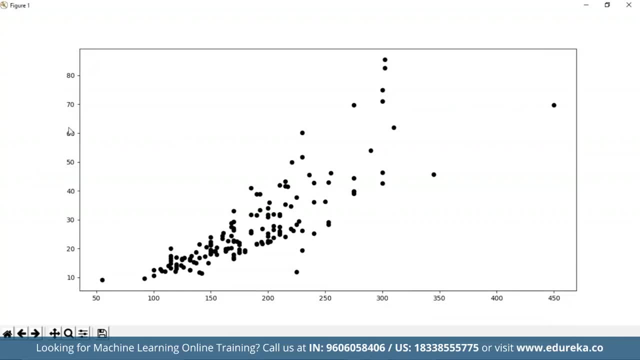 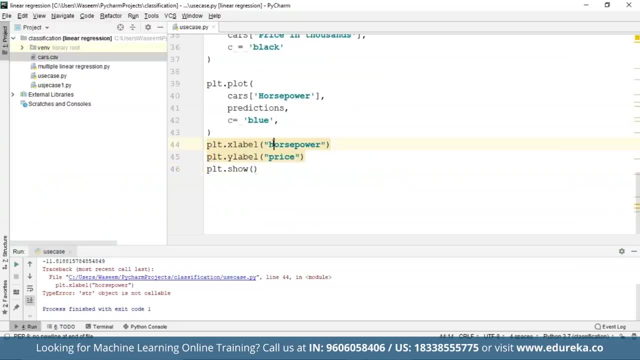 450 horsepower, and this is actually our price. Now when I close this: Okay, I've made a mistake somewhere. Okay, this is actually Now when I run this again. I should be fine. I close this and after this: Okay, so I've got the mistake that I was making. 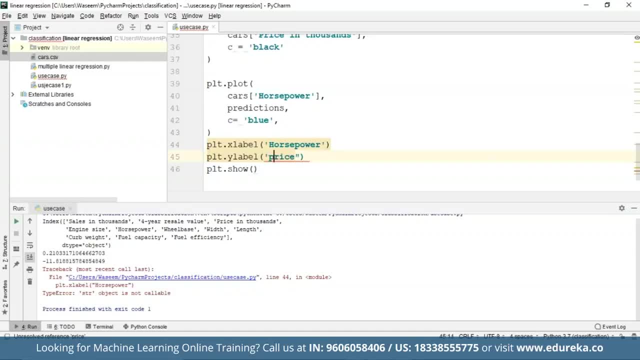 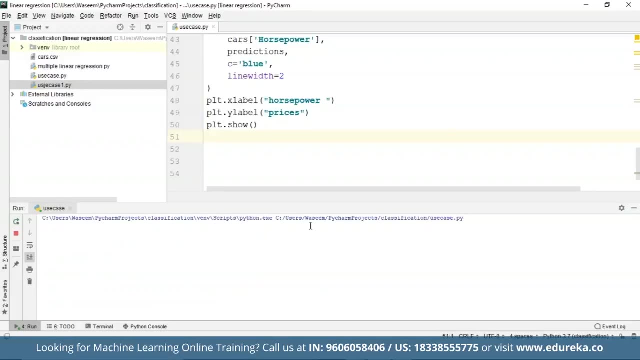 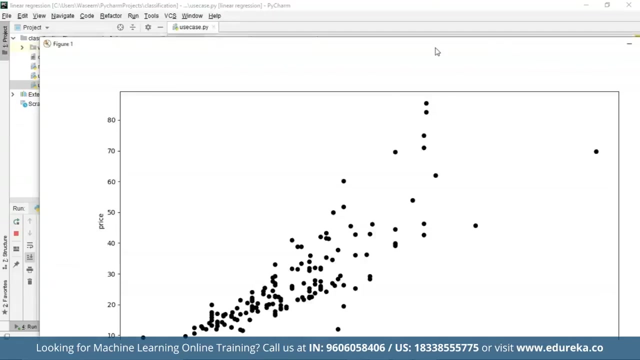 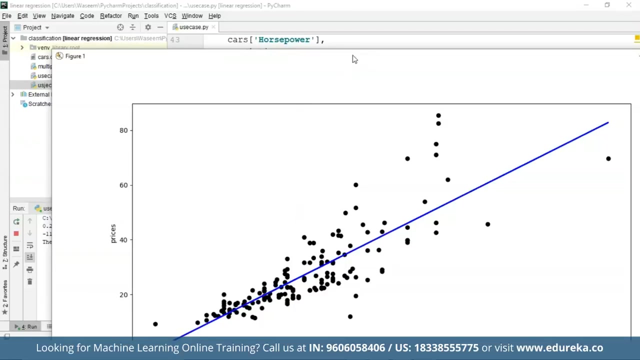 So before running this program, I'll add the line width as well, And let's just run this again. So first I'm getting this, which is horsepower, right here, and we have the price right over here. After this, Let's see. So we have a best-fit line over here, as you can see, guys. 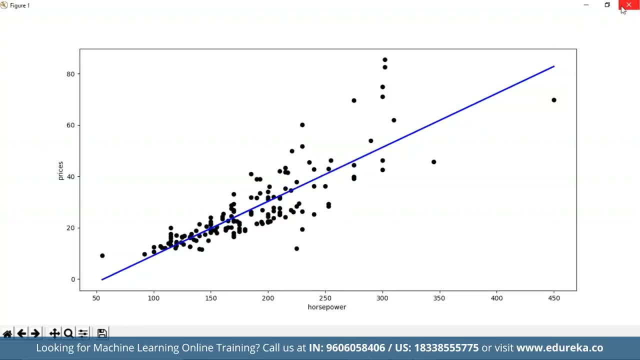 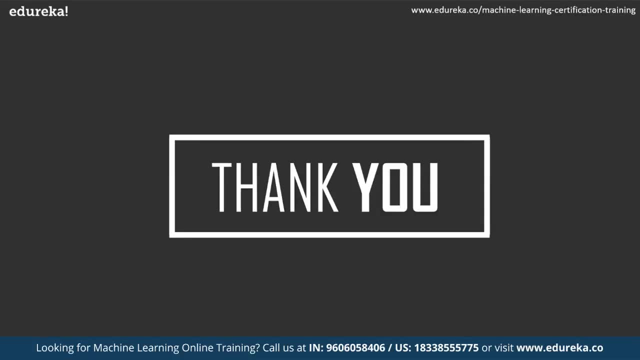 So this is a simple linear regression implementation on a custom data set. So now that we are done with our use case as well, Don't forget to subscribe to your director for more exciting tutorials, and also press the Bell icon to get the latest updates from Eddie Raker. also do check.